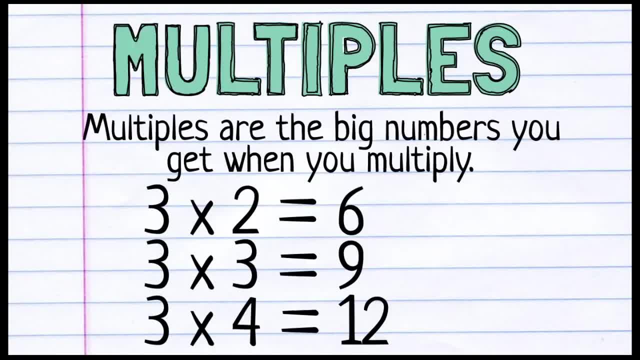 What are multiples? Multiples are the big numbers you get when you multiply. So here we see: 3 times 2 equals 6, 3 times 3 equals 9, 3 times 4 equals 12.. These numbers, these are multiples of 3.. 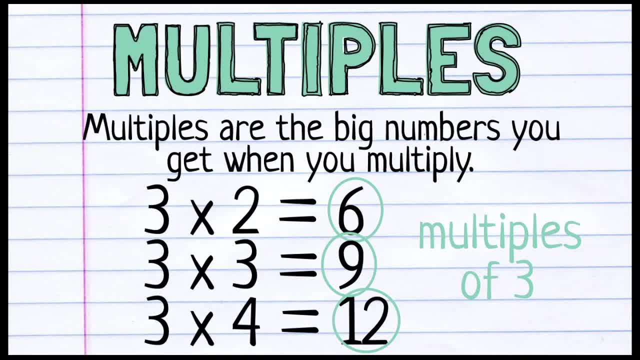 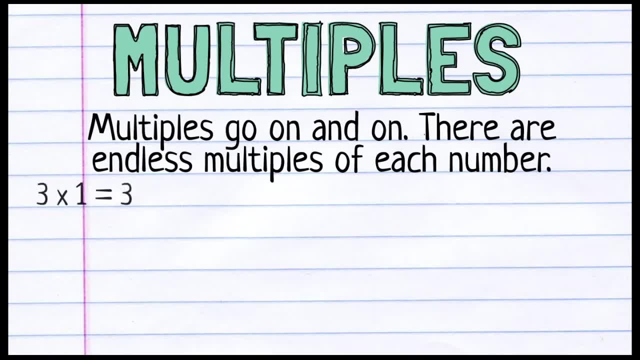 When I multiply 3 by something, I get a multiple of 3.. And multiples can go on and on. There are actually an endless number of multiples for each number. So when I multiply 3 by anything, I'm going to end up with a multiple of 3.. 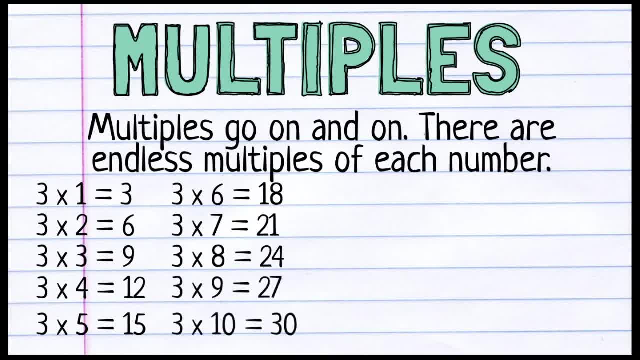 3 times 6,, 3 times 7,, 3 times 8,, 3 times 9,, 3 times 10.. We can keep going, multiplying 3 by bigger and bigger numbers. each time, And every single time, we will end up with a multiple of 3.. 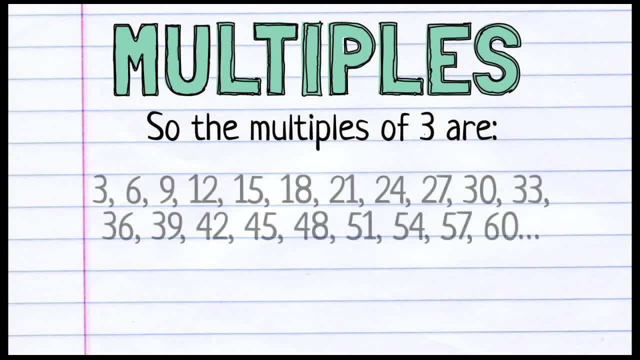 So what are the multiples of 3?? 3,, 6,, 9,, 12,, 15,, 18,, 21,, 24,, 27,, 30,, 33,, 36,, 39,, 42,, 45,, 48,, 51,, 54,, 57,, 60. 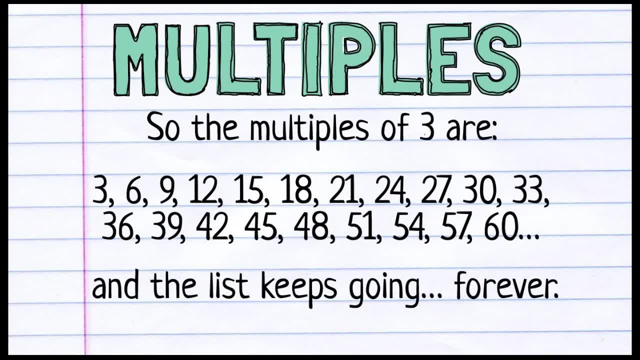 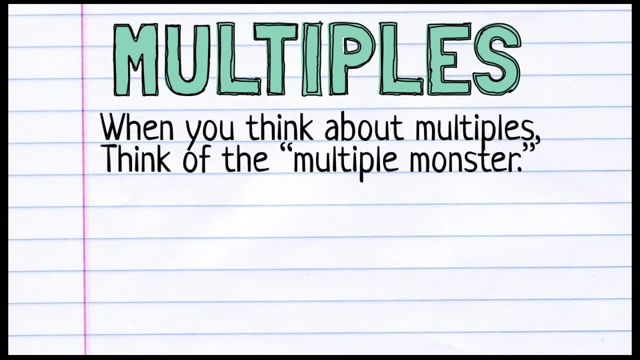 These are all multiples of 3.. And the list keeps going forever, Literally forever. You could list multiples of 3 until the end of time. There is an infinite number of multiples for each number. When you think about multiples, think of the multiple monster. 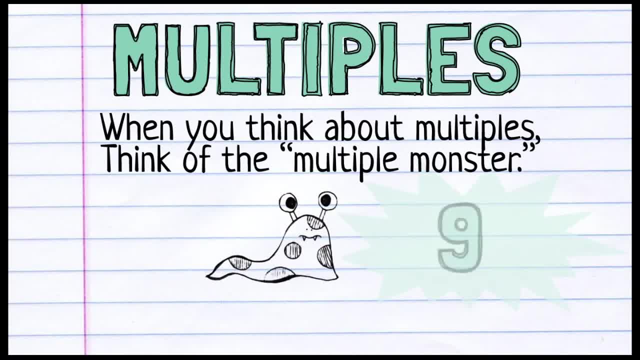 So the multiple monster makes numbers bigger. Each time you list a multiple of 3, the number is getting bigger and bigger and bigger, And it's actually increasing by the number itself Each time. it's going up by 3.. So the multiple monster makes numbers bigger. 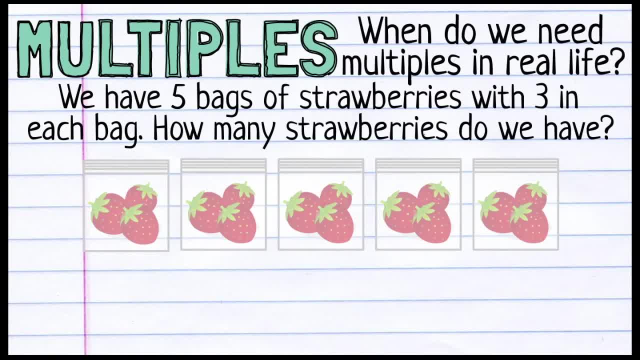 So why might we need to know about multiples? Why do we need to use multiples in real life? Let's say we have a bag, We have five bags of strawberries And there's three strawberries in each bag. How many strawberries do we have? 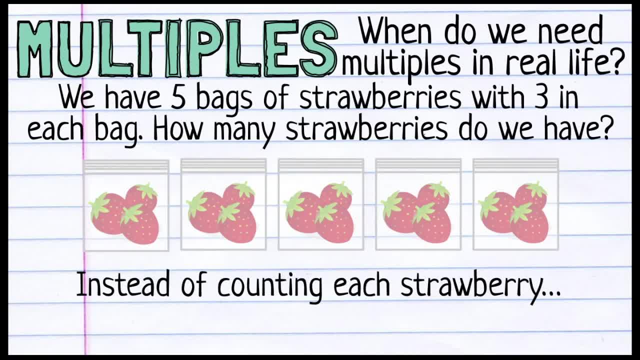 Well, instead of counting each strawberry: 1,, 2,, 3,, 4,, 5,, 6,, 7,, 8,, 9,, 10,, 11,, 12,, 13,, 14,, 15.. 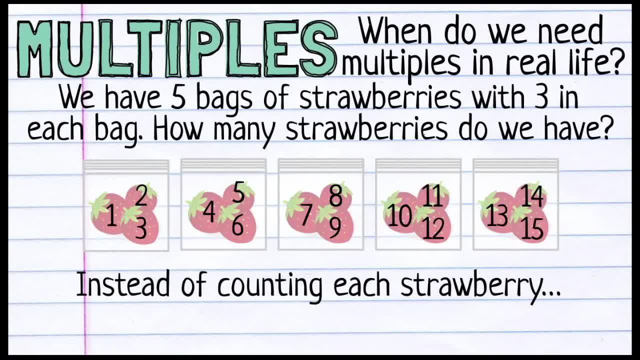 That's just not a very efficient way to count the strawberries. We have a better way because we know about multiples. We can use Multiples to count groups of three like this: 3, 6,, 9,, 12,, 15.. 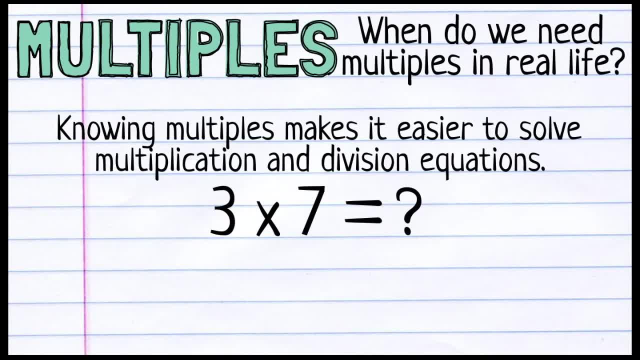 Multiples can also make it easier to solve multiplication and division equations. If I'm trying to figure out what 3 times 7 is, I can just list multiples of 3. When I list them out, I'm looking for which multiple is the seventh one on the list. 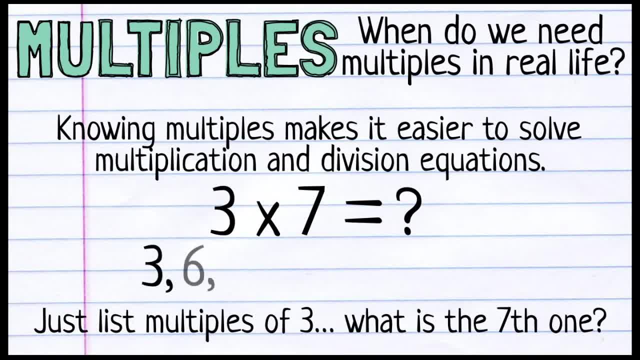 Let's find out 3.. That's the first multiple of 3.. 6 is the 7th one. That's the 2nd one. 9.. That's the 3rd one. 12 is the 4th multiple on my list. 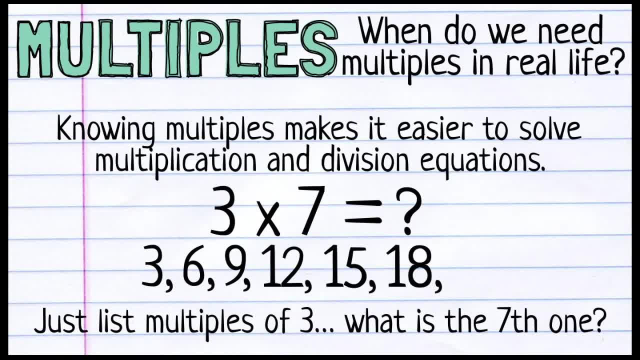 15. That's the 5th one, 18 is the 6th multiple of 3. And 21.. 21 is the 7th multiple on my list when I listed out multiples of 3. And that means that 3 times 7 is 21.. 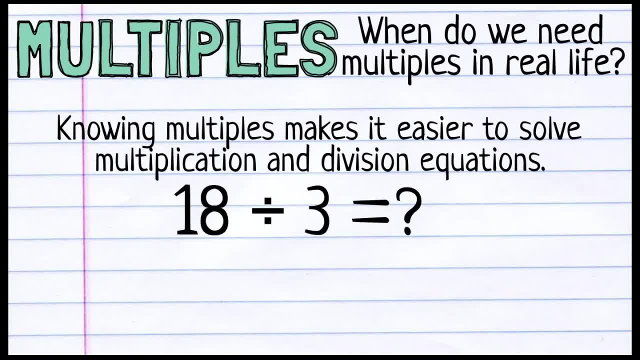 This also works with division equations like 18 divided by 3.. This time I'm listing multiples of 3 and I'm trying to figure out when I hit 3.. When I hit 18, what multiple is that? What number multiple on my list like this: 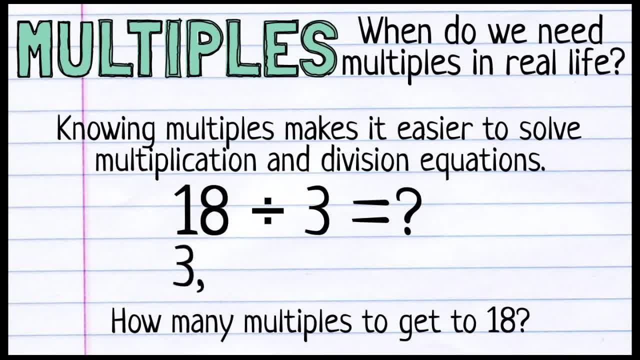 3.. That's the first multiple, So that's 1,, 2,, 3,, 4,, 5,, 6.. Oh look, there's 18.. 18 is the 6th multiple on my list of multiples of 3.. 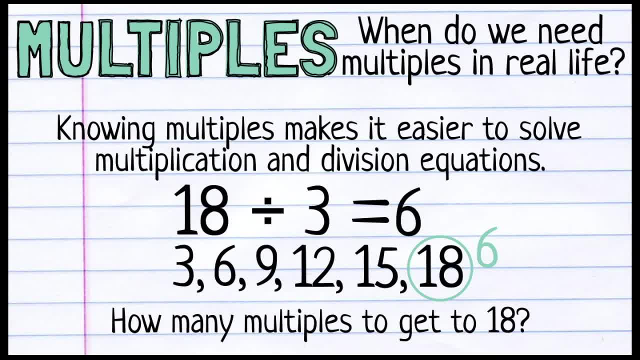 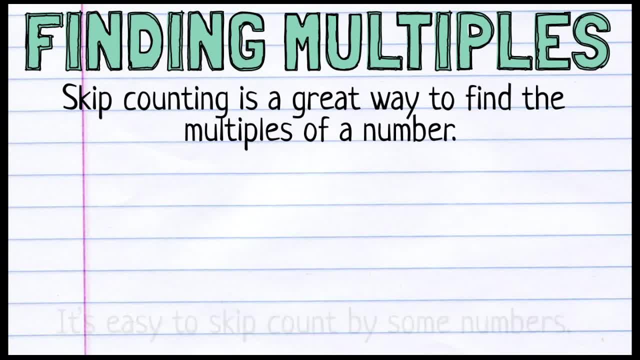 So 18 divided by 3 is 6.. So how do we find multiples? Well, skip counting is a great way to find the multiples of a number And some numbers are really easy to skip. count by like 2.. It goes like this: 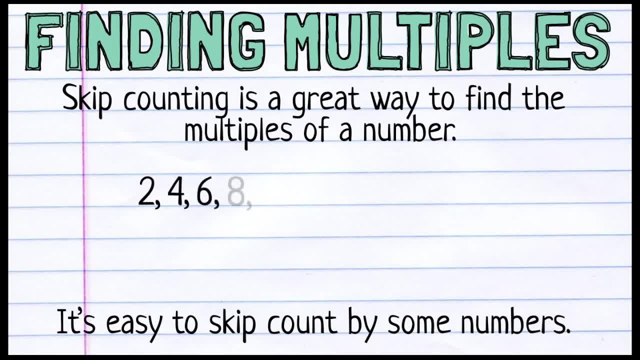 2,, 4,, 6,, 8,, 10,, 12,, 14,, 16,, 18, 20.. You've probably been counting by 2's. since you were very small, It's also easy to skip count by 5's. 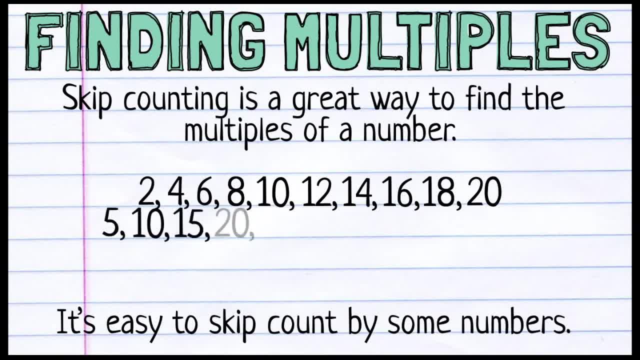 5, 10, 20.. 15,, 20,, 25,, 30,, 35,, 40,, 45,, 50. These are multiples of 5. When you are skip counting by a number, you're listing the multiples of that number. 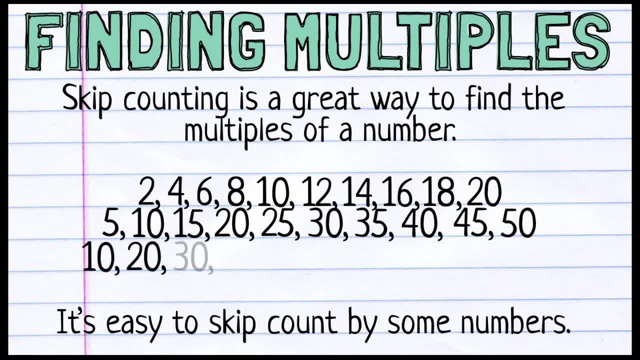 10 is another easy one: 10,, 20,, 30,, 40,, 50,, 60,, 70,, 80,, 90,, 100.. I could keep going: 110,, 120,, 130.. 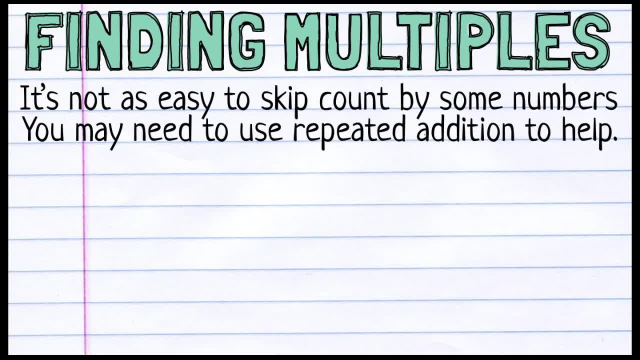 These are multiples. Now some numbers are not as easy to skip count by, So you may need to use repeated addition to help you. Let's try skip counting to list the multiples of 6.. Hmm, I can't count by 6's as easily as I can count by 2's, 5's and 10's. 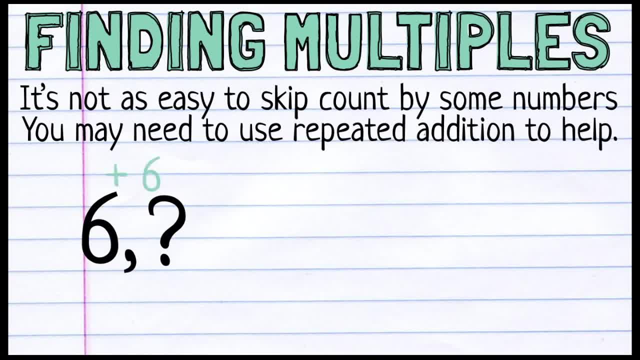 So I may need to use addition here. Let's just think about adding 6 more 6 plus 6 is 12.. So that's the next multiple on the list. Okay, This is the first multiple on the list. What would come after 12?? 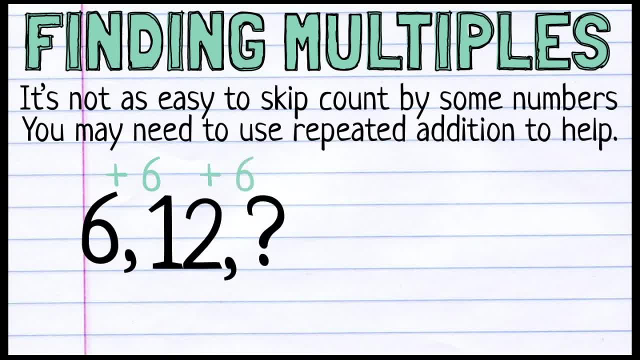 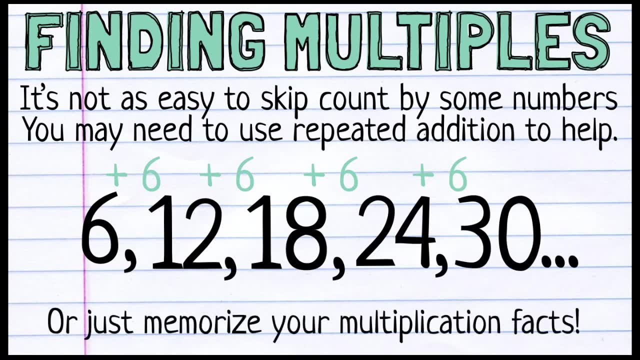 Well, let's add 6 again. 12 plus 6 is 18.. Let's add 6 again to get the next number: 18 plus 6 is 24.. 24 plus 6 is 30. And I could go on and on. 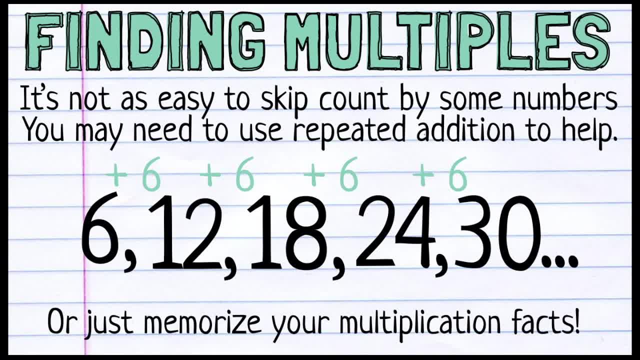 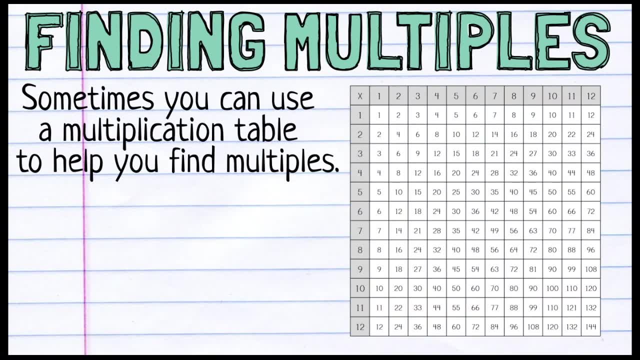 You can see this is kind of a lot of work. So really it's best to just memorize your multiplication facts Will do six facts memorized, you won't have to bother with all of this. add six, add six, add six- nonsense, you'll just know the multiples of six. sometimes you can use a. 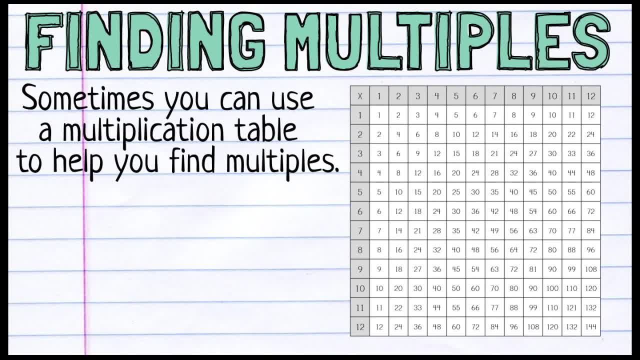 multiplication table or a multiplication chart to help you find multiples. so the multiples are actually on here twice. you can see here highlighted the multiples of one. they go over and also up and down, so they're in rows and columns. those are multiples of one, multiples of two, multiples of three, multiples of four.